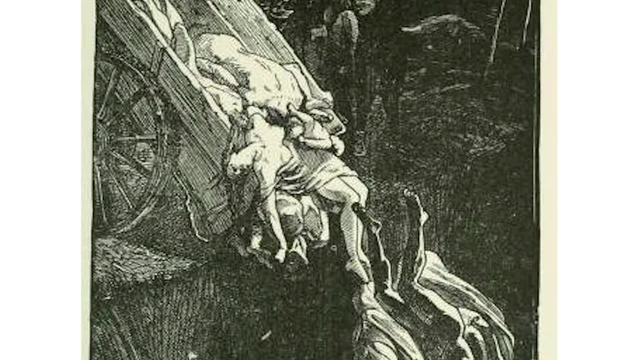 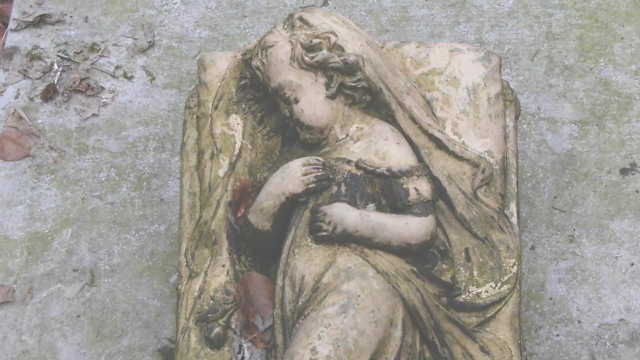 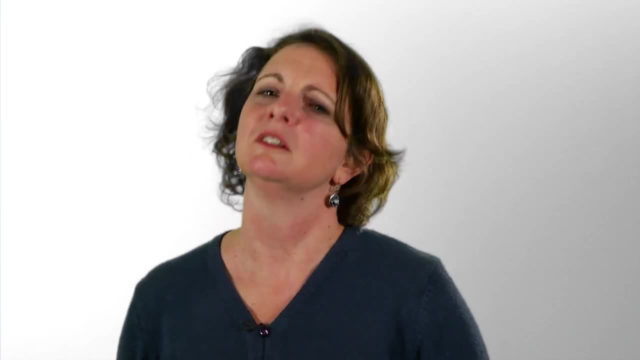 were really high Because of things like the plague, famine, war and poor living conditions. people died pretty young. To make up for all those people dying, they had to have a lot of babies. Of course, there were other reasons too. I'm sure you can imagine a few. First, we need to recognize 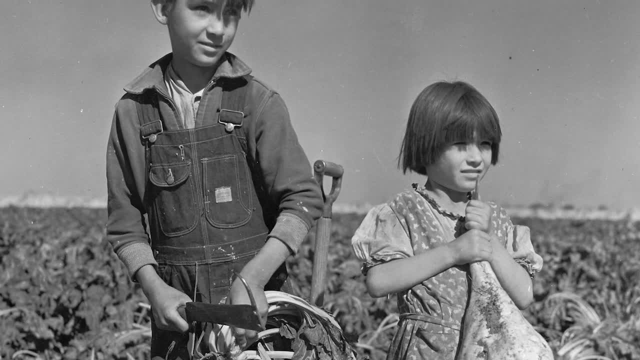 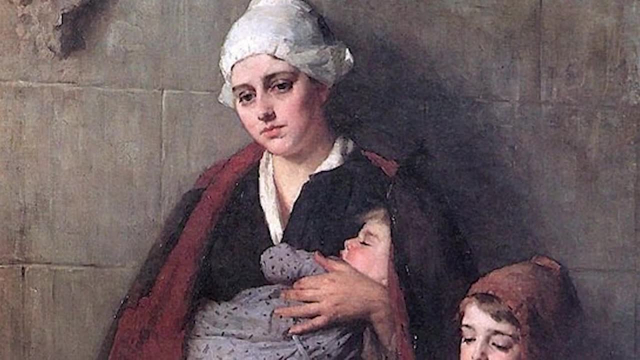 that children were defined as assets. They were workers, of course, usually helping their families with different tasks. A woman's status was also defined by how many children she had, especially if they were boys, And these women and children were seen as property. 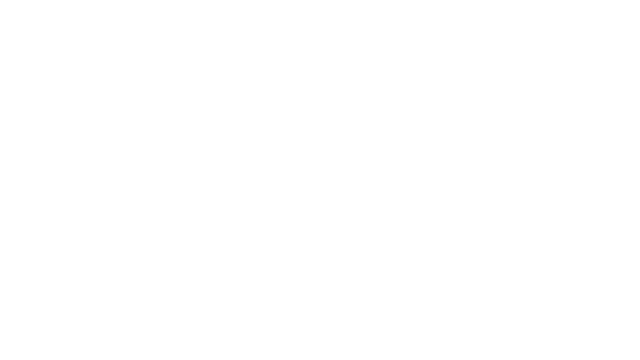 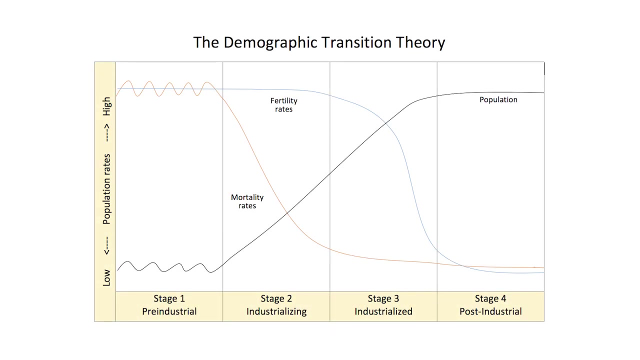 and therefore represented the wealth of men. They also would want to make sure that enough children would live long enough to take care of them when they were old, Throw in religious and cultural norms, and you can see why the fertility rates were so high. 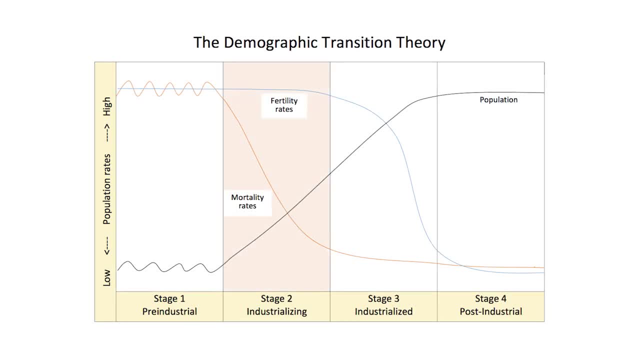 Then something shifted. You can see that beginning in 1750, with the start of the Industrial Revolution, that mortality rates began to drop. The early industrial era of stage two is marked by improvements in sanitation and health care. But notice that the fertility 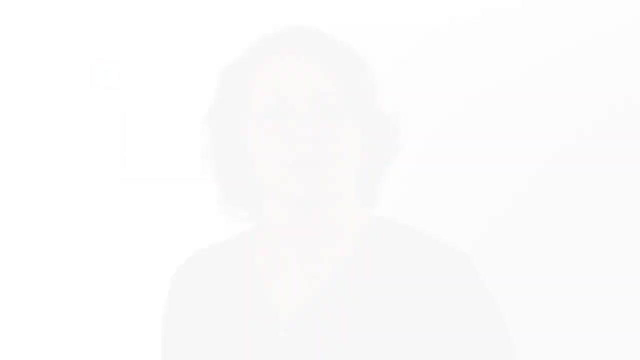 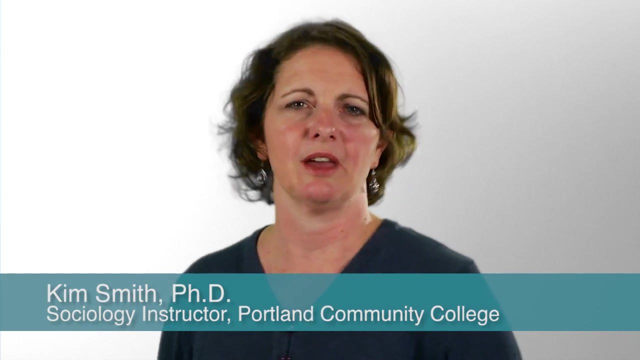 rates stay high. This is known as a cultural lag, because the technology that improved mortality rates changed faster than the culture's ability to adapt. Think about it: How long would it take to simply have faith that your babies would live, so you didn't have to have so? 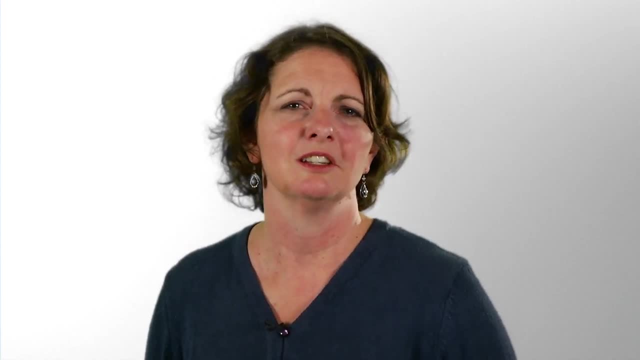 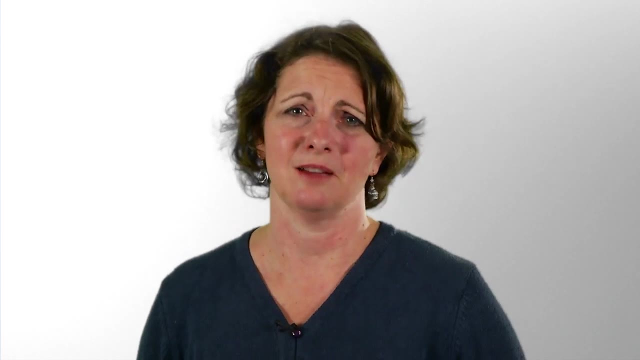 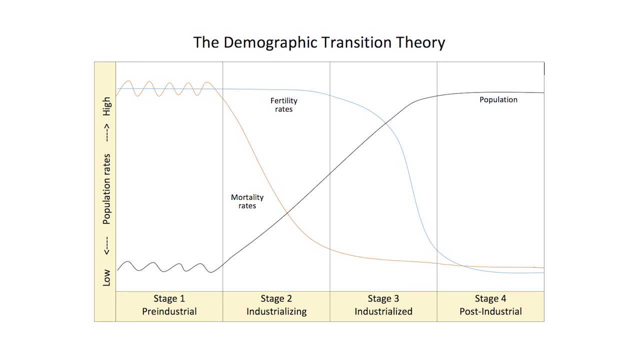 many: One, Maybe two generations. What about the time it would take to change gender roles or religious norms? Well, that's a long time, And over that time, look what's happening to the population level. Just do the math. If fertility rates stay high and mortality rates are low, then the 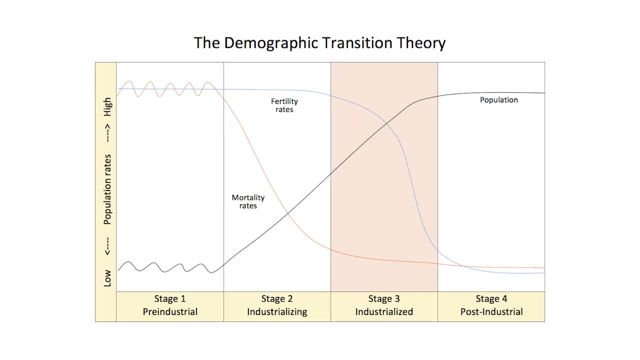 population booms, Note that by stage three, as industrialization continues, the fertility rates eventually start to drop. One of the biggest reasons for this is that children are redefined from assets to liabilities. While most people still want to have children, they choose to have far fewer than in the past. Beyond decreasing child mortality and 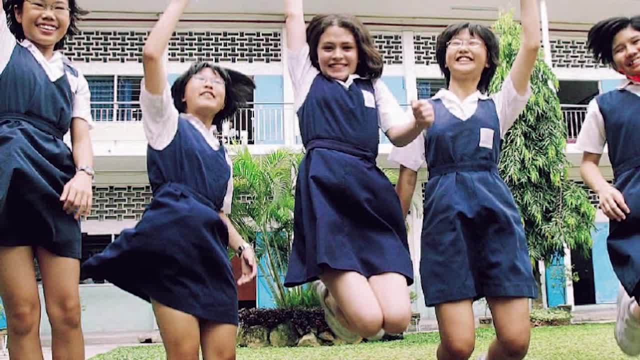 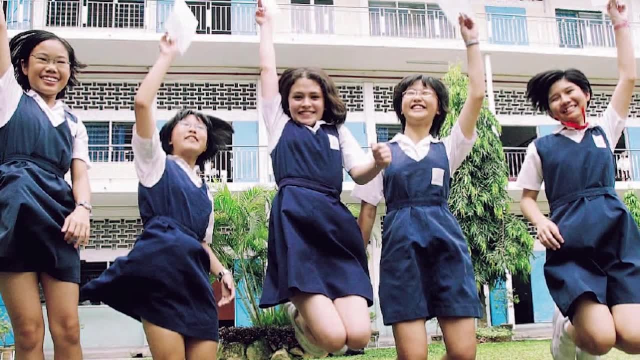 changing elder care. they choose to have far fewer than in the past, Beyond decreasing child mortality and changing elder care. girls are going to school, women are working and most industrialized countries have child labor laws, So bottom line women are postponing having children. Plus, kids are expensive. So fertility rates in industrialized countries continue to drop and are now close to, if not below, replacement rates, Thus, by stage four, in post-industrialized countries mortality and fertility rates are both low and population booms And population growth finally stabilizes again. This looks pretty good, right, Well there. 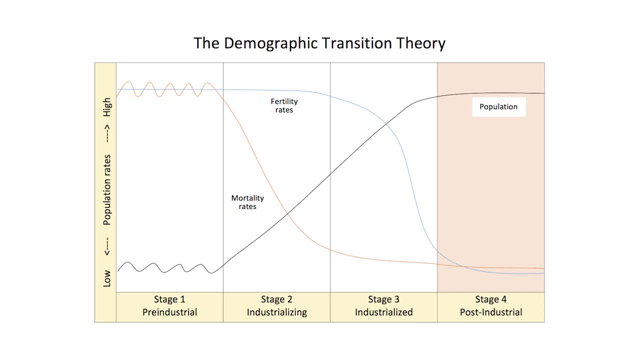 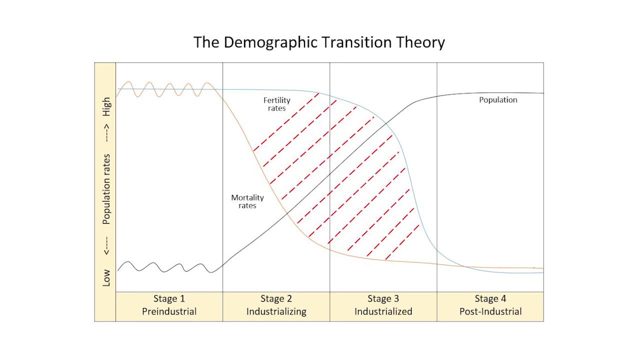 are some caveats. First, there's a big risk. What about this stage in the middle where the fertility rates are so much higher than mortality rates, With all of this population growth? Lester Brown warns us about the risk of the demographic trap Instead of transitioning. 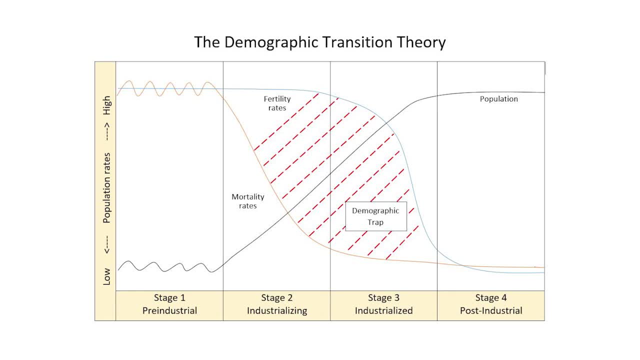 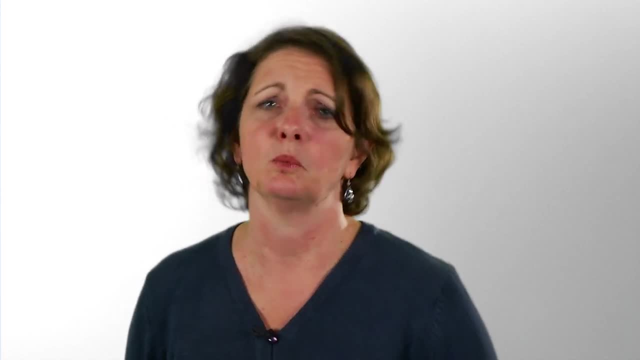 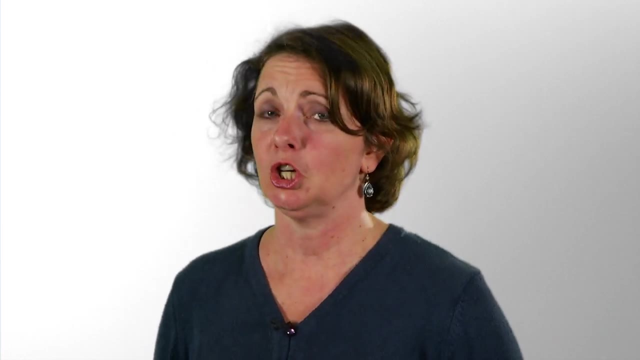 into stage three and four. a region can get overwhelmed by people and go beyond its carrying capacity. In that case, food and water and other necessities will run out. In fact, things could get so bad that they will consume all of their resources and mother nature, and 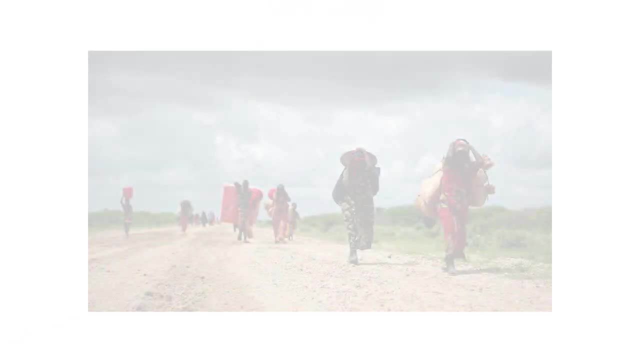 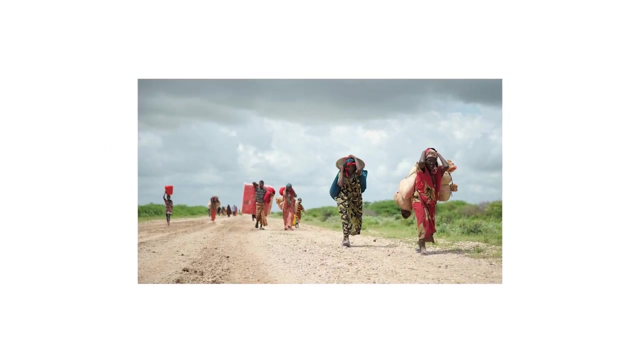 human conflict will push them back into stage one. It's not a pretty picture, and mother nature can be very harsh. We're already seeing this happening in different regions around the world, such as in Somalia, where environmental problems are becoming the number one cause of refugees. But that's. 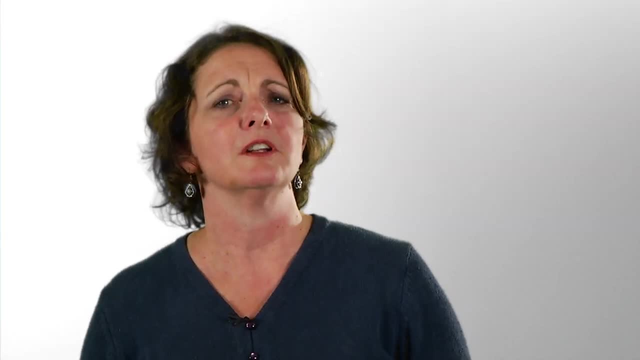 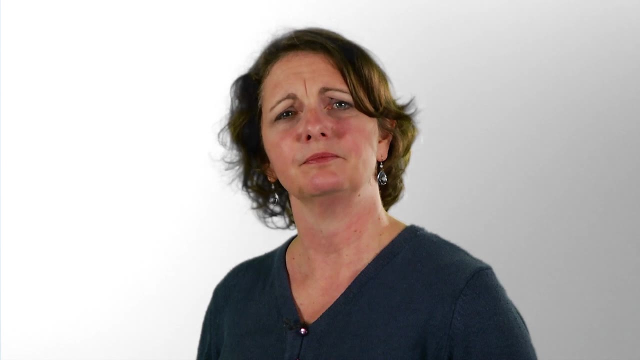 not the only risk. While some policy analysts, who are often called anti-Malthusians, believe that the answer to overpopulation is industrialization and economic development, because that is what has worked in the past, others warn that there simply aren't enough resources. on the 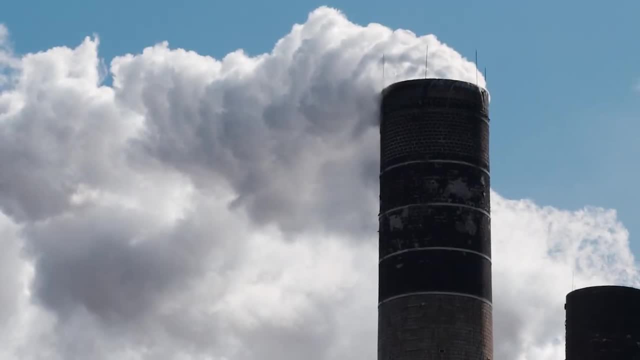 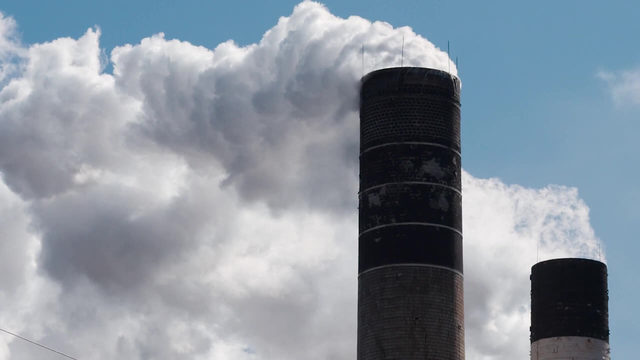 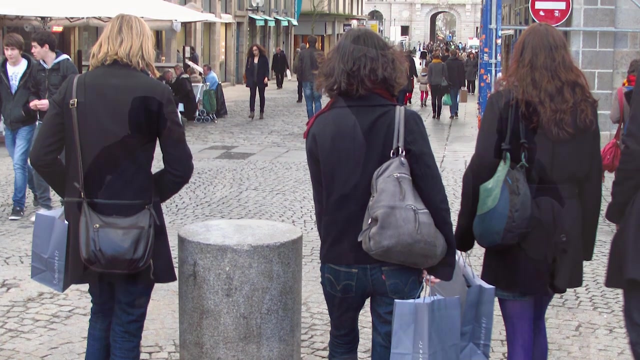 planet to enable countries all around the world to industrialize in the manner of the past. These neo-Malthusians, who base their assumptions on the teachings of Thomas Malthus, critique the demographic transition theory because they claim that the consumption of the industrialized world faces very real limits on a finite planet. 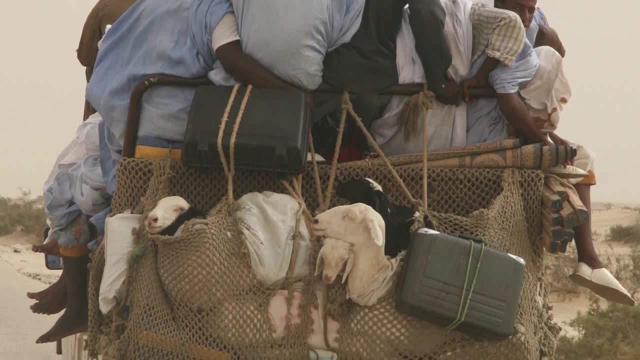 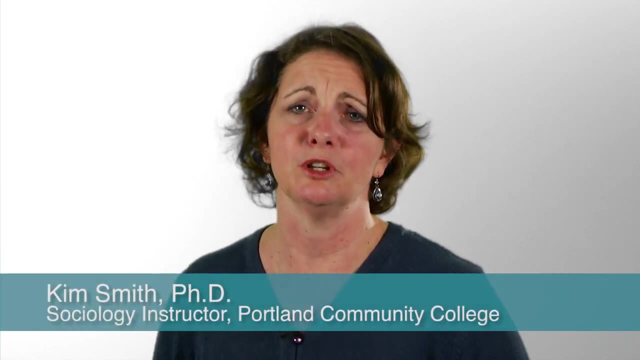 While we certainly have solved a lot of problems with science, technology and economic development, and it is argued that there currently is enough food on the planet if we had proper distribution, it is still unclear if industrialization is the answer to overpopulation, given our consumption.